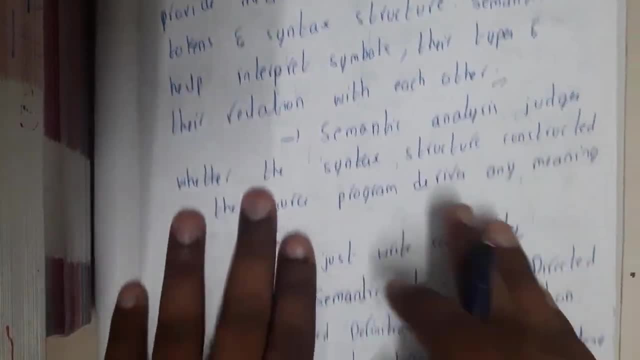 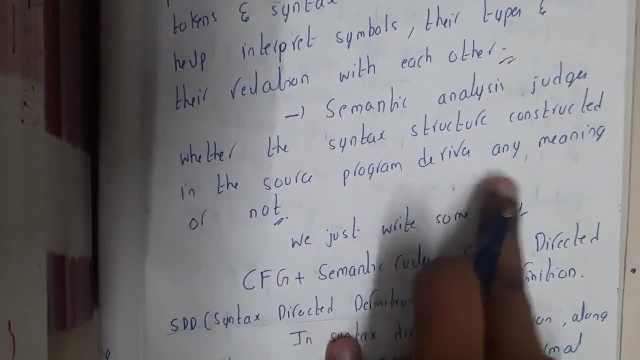 checking and all those things will be done in this semantic analysis only, guys Okay. So semantic analysis judge whether the syntax structure constructed in the source program derives any meaning or not. So whether it is meaningful or not, it is checked here itself, guys Okay. 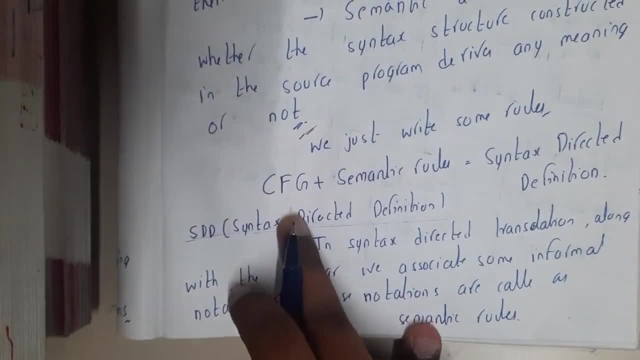 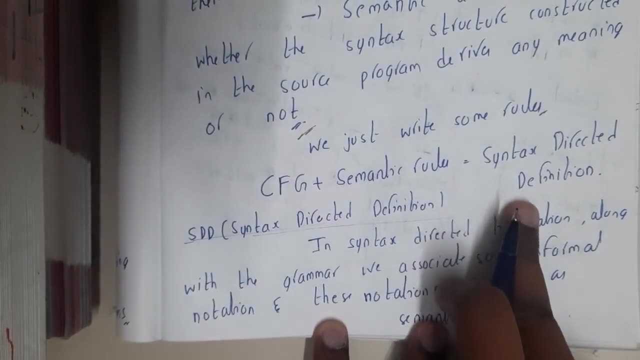 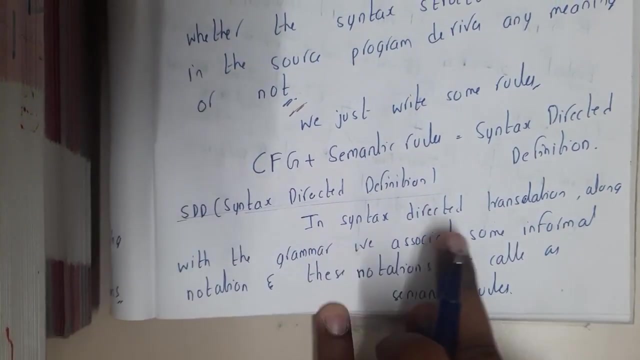 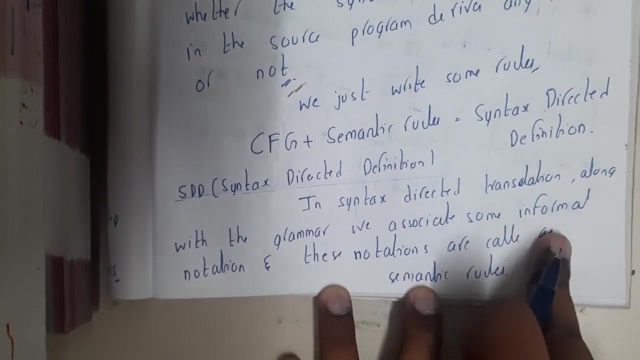 So we just write some rules. The rules is: specify about context-free grammar plus a semantic rules is equal to syntax directed definition, guys, Okay. So SDD is equals to syntax directed definition. Okay. So in syntax directed definition translation, along with grammar, we associate to some informal notations, and these notations are called as semantic rules. 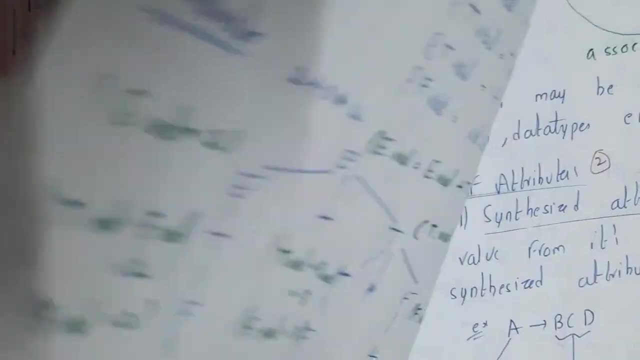 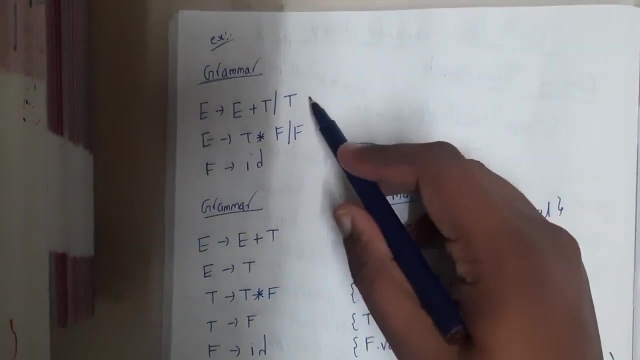 Guys, once we are going through an example, you will be having a clear idea about it, guys. So don't worry, Okay. Okay, So the grammar is defined as a semantic structure, So semantics is defined as a grammar. So if you take a grammar in this way, so E. 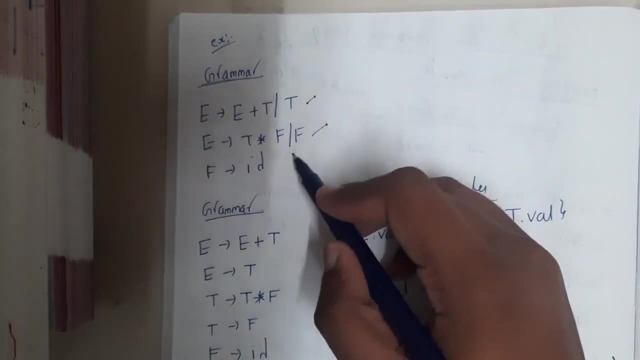 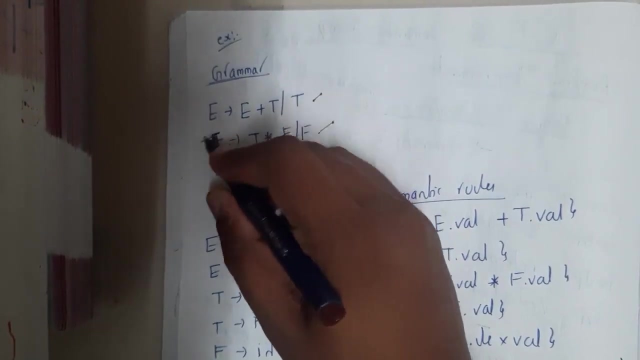 implies an E plus T or T. E implies E into T or T. E implies ID. Sorry, F implies ID. Okay, So I think it should be T, right So, rather than E, Okay. So E implies E plus E. The semantic rule will be E dot val. 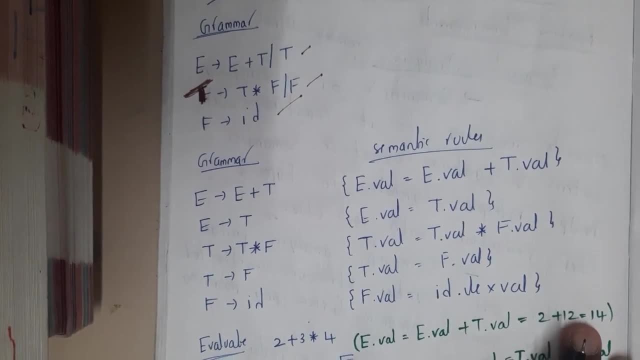 is equals to E dot val plus a T dot val. Simoneally, E dot val is equals to T dot val. Similarly, T dot val is equals to E dot val in this text, Right. So it is just not enough to 봤ing it and deriving the way You can see theesser. it becomes a factorial that is effective on several of its authorities. so what we have actually, it is not that simple one, right. Suppose you want to safely accept it, then why it should actually take? so if we take 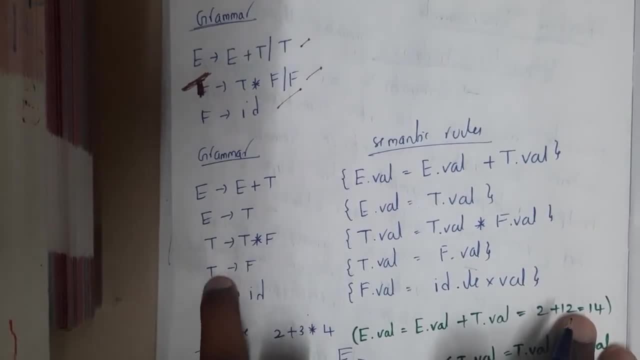 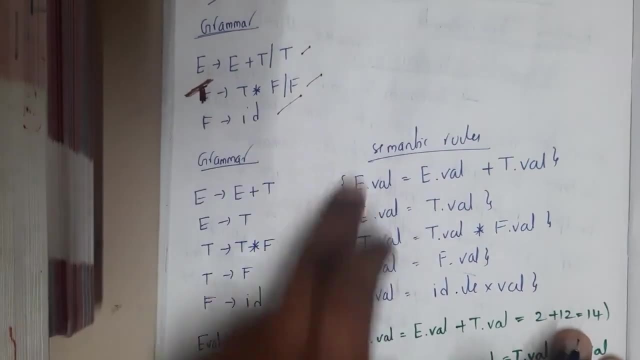 val is equals to t dot val into f dot val: t dot val is equals to f dot val. f dot val is equals to id dot lex val. so these are the semantic rules, guys. i have just told you right now. okay, yes, just by observing the grammar you can say them. there are. there is nothing special in it, guys, so dot. 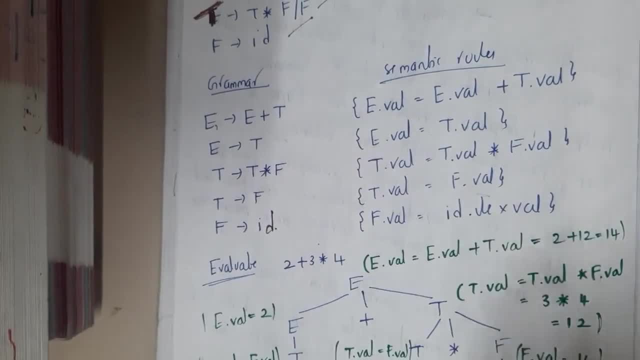 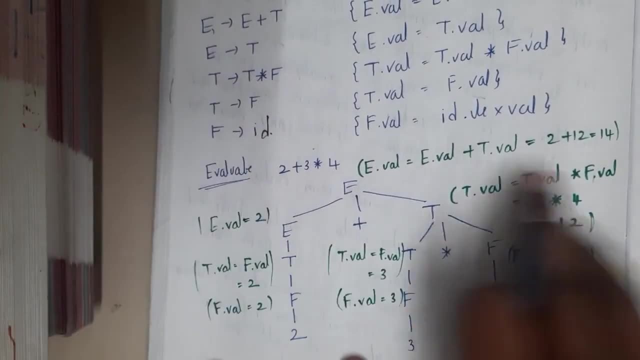 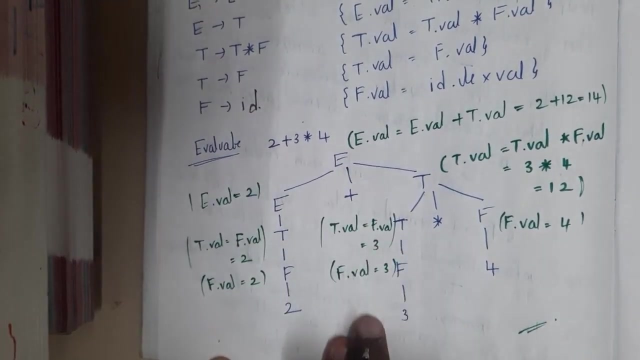 value you will be adding, and for identify- sorry for any kind of, any kind of terminal- you will be writing dot lex val. that's it. so e evaluation, so evaluation for the function, for the expression 2 plus 3 into 4. it will be in this way, guys. so you will be writing: e implies e plus t and t. 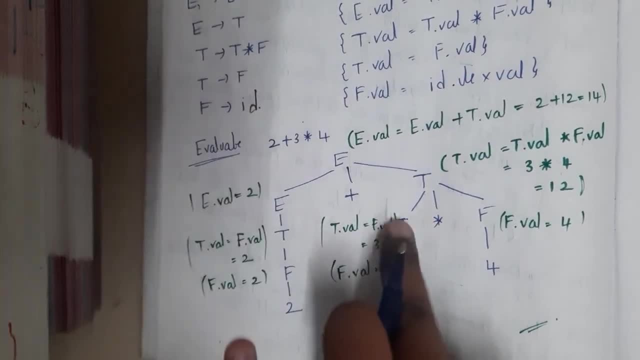 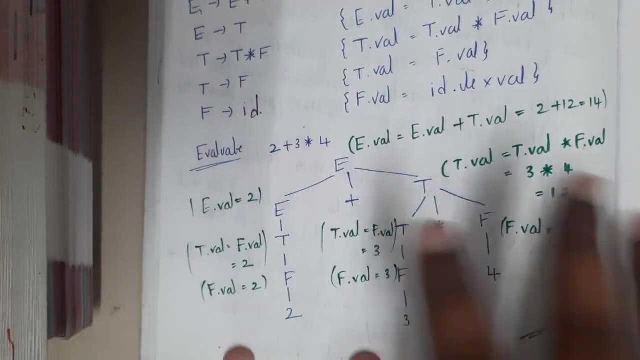 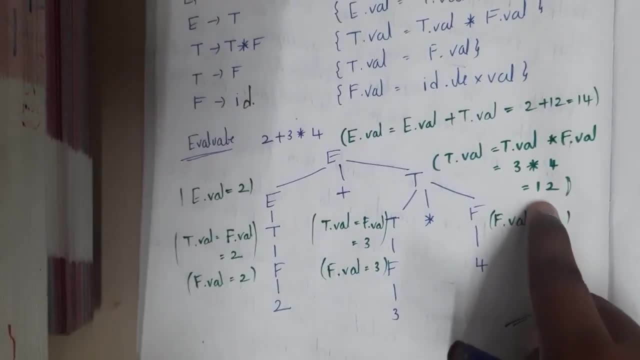 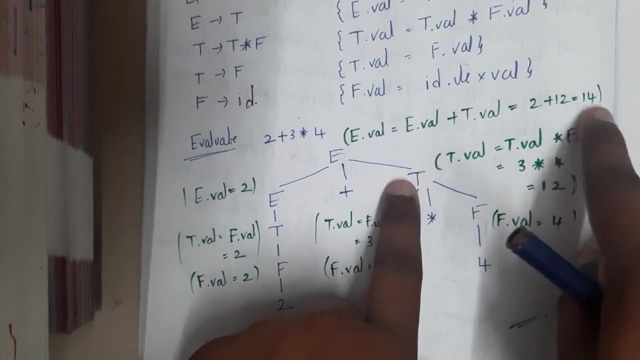